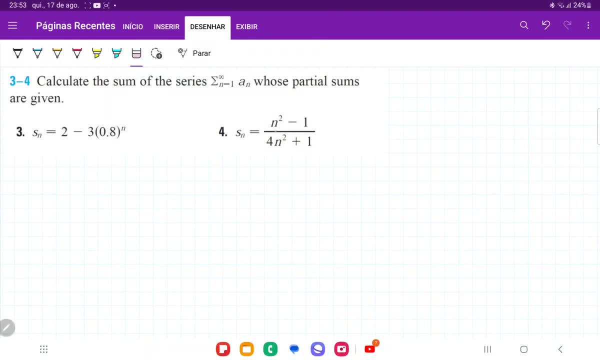 So for number four, we want to calculate the sum of the series whose partial sum is given. So this is the partial sum, And so what this means is that we have the sum of some sequence- a, n. we don't know what that sequence is, and we're summing it from one to infinity. 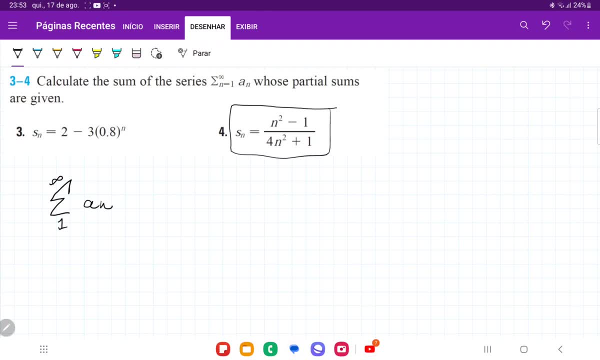 And so when we sum it, we get a sequence of partial sums right. So the sum, say, of 10, it's going to be the sum of a 1, a 2, a 3, a 4, and so on until a 10.. So we have that the sequence. 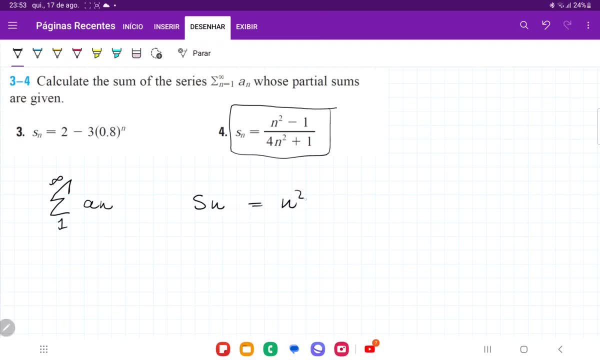 of partial sums is given by n squared minus 1 over 4n squared plus 1.. So what this means is that suppose that I want the sum from 1 to 10.. All I have to do here is plug 10 for n and I'm going. 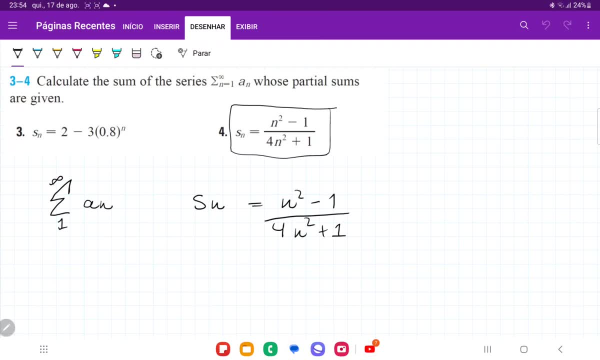 to get the sum from 1 to 10, right of all the terms. So it wants us to see what the sum is if we sum from 1 all the way out to infinity. So in practice we are summing up infinite terms. So what we have to do here is: 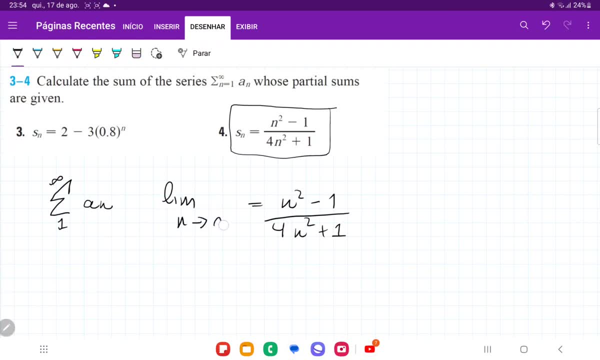 we have to take the limit as n approaches infinity of this guy over here, Because if we take this limit it's like seeing what happens to the sum as we add infinite terms And so if we just take this limit over here it's going to give us infinity minus 1 is infinity over 4 times infinity. 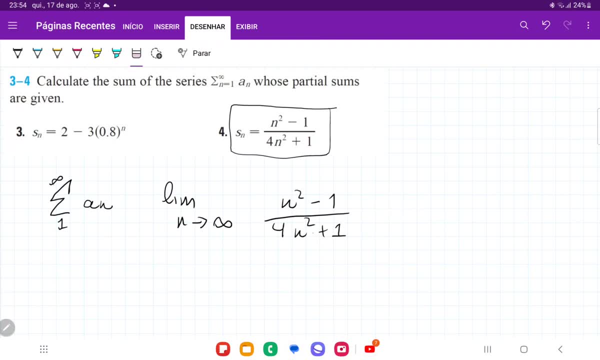 squared, So that's going to be infinity And that doesn't really help. So what we're going to do is we're going to divide by the highest coefficient. So we're going to divide everything by n squared, So 1 over n squared on the top. 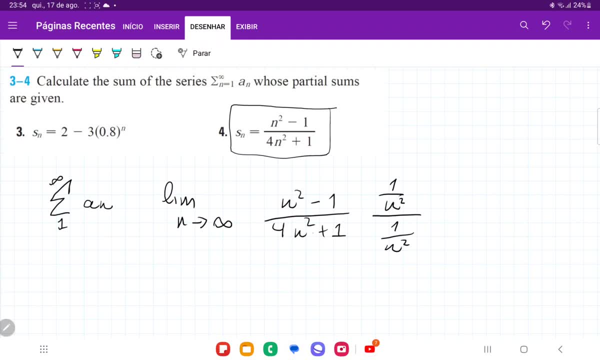 and 1 over n squared on the bottom. And the reason that we're doing this is so that we can at least get some numbers. We're going to get rid of the infinity right And we're going to have infinity in a quotient. And a quotient is really nice because whenever we're dividing by infinity, 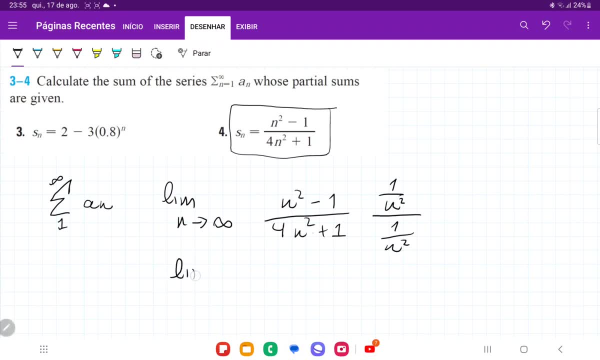 it goes to zero, And so this is the same thing as the limit as n approaches infinity. of n squared divided by n squared is 1 minus 1 over n squared 4. n squared divided by n squared is just 4.. And then plus 1 over n squared. So